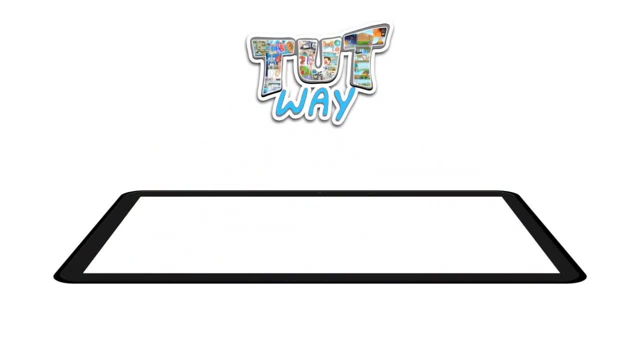 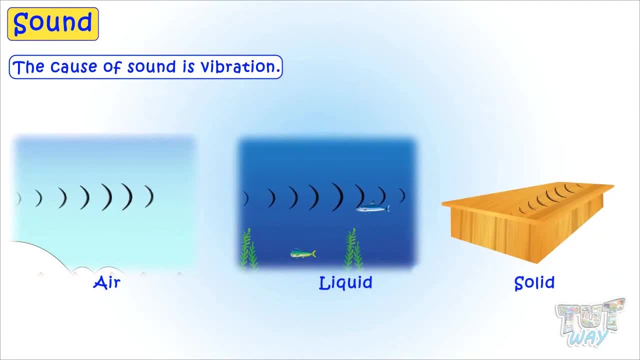 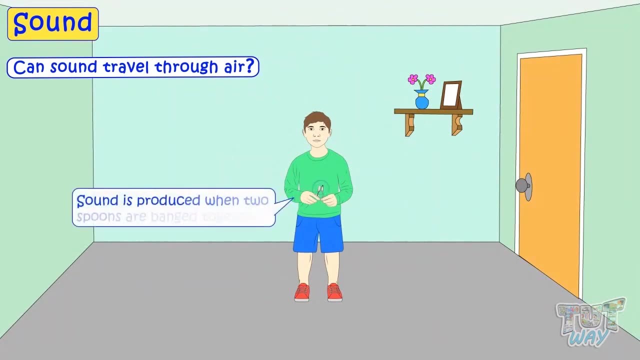 TootWay has thousands of animated videos on math, English and science. TootWay has thousands of animated videos on math, English and science to clear the core basics of these subjects. Let's see, can sound travel through air? Take two spoons and bang them together. 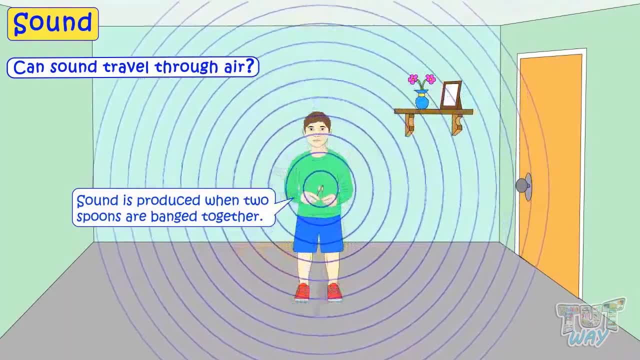 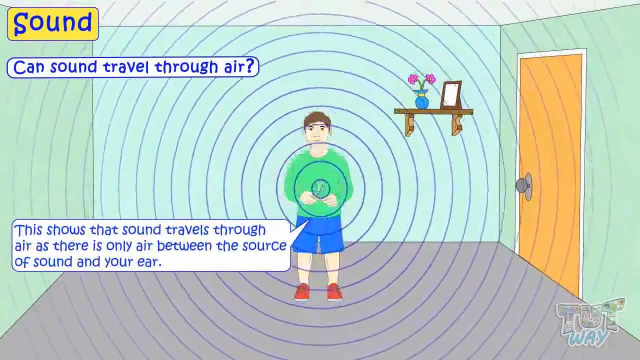 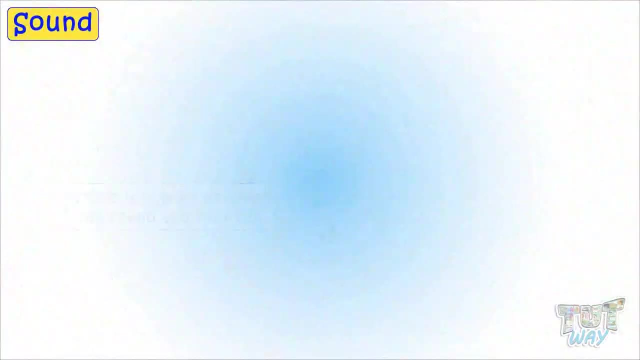 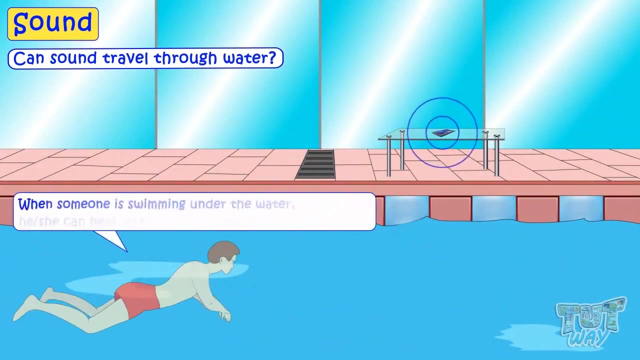 You hear the sound. It shows that sound travels through air, As there is only air between the source of sound and your ear. Now let's see. Can sound travel through water When you are under water or when someone's swimming under the water? 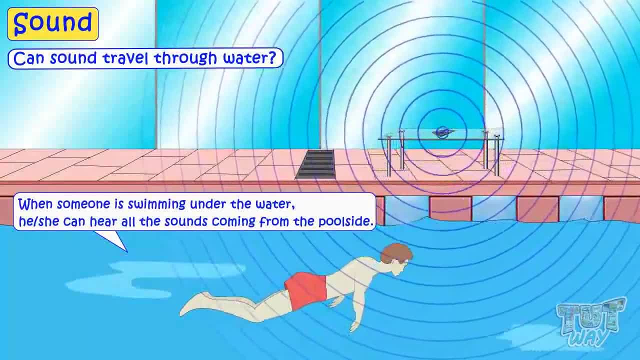 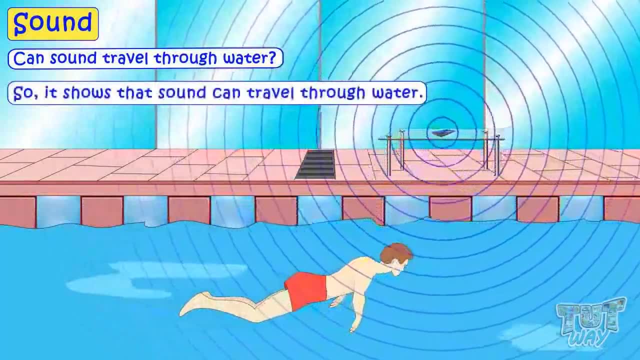 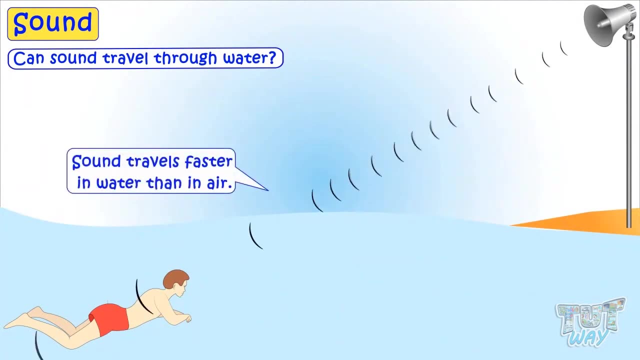 he or she can hear all the sounds coming from the poolside, So it shows that sound can travel through water Rather. sound travels faster in water than in air. Divers can listen to every sound That is coming from outside the water. 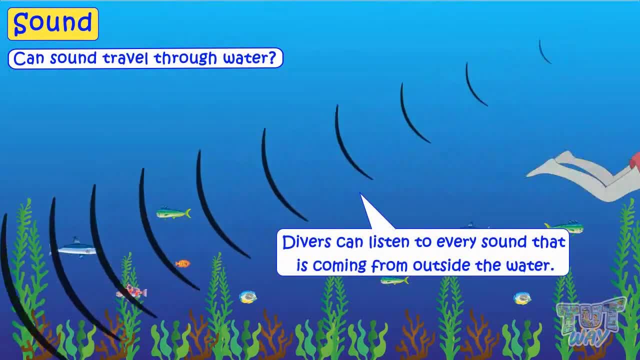 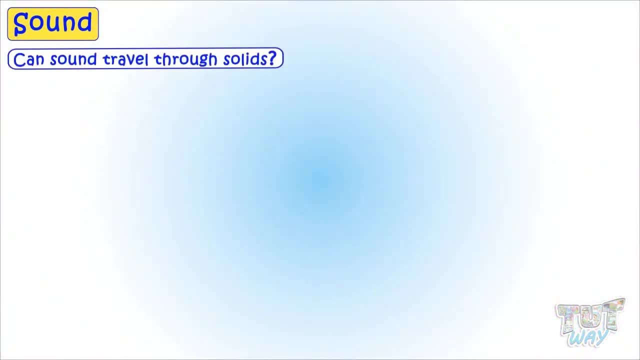 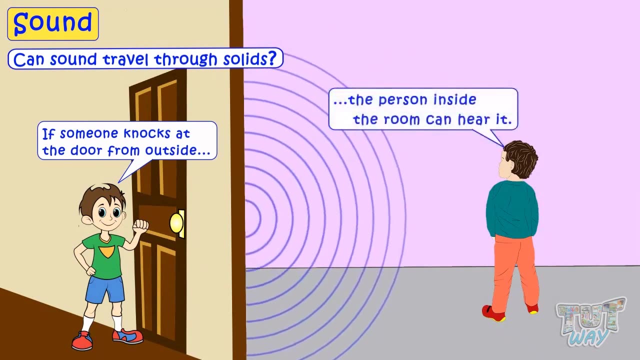 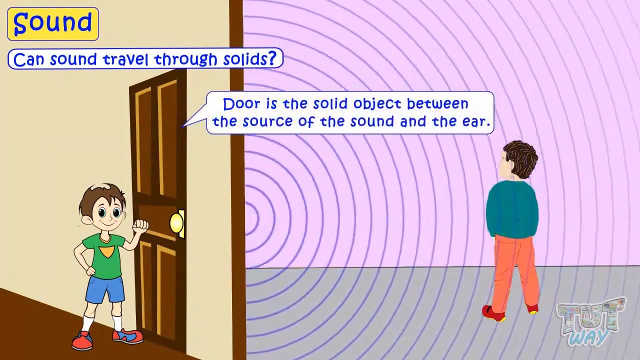 This shows that sound waves can travel through water. Now let's see if sound can travel through solids. If someone knocks at the door from outside, the person inside the room can listen And there is a solid object, that is a door between the source of the sound. 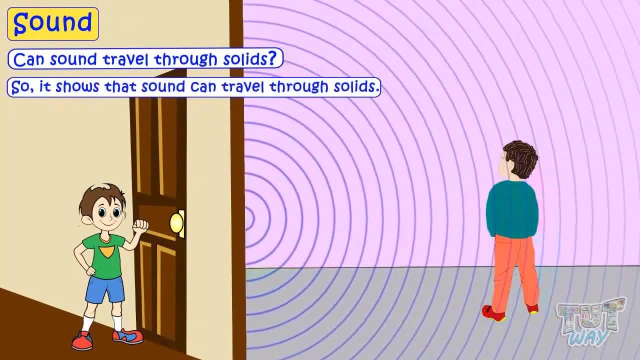 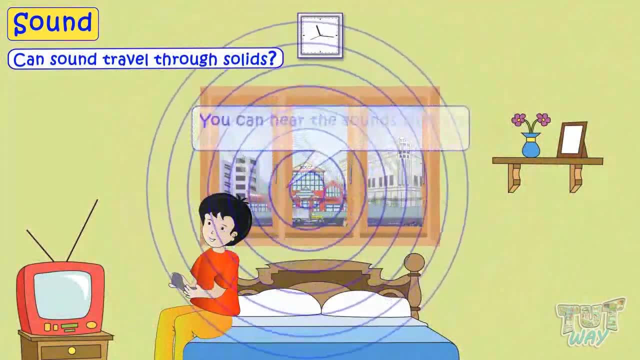 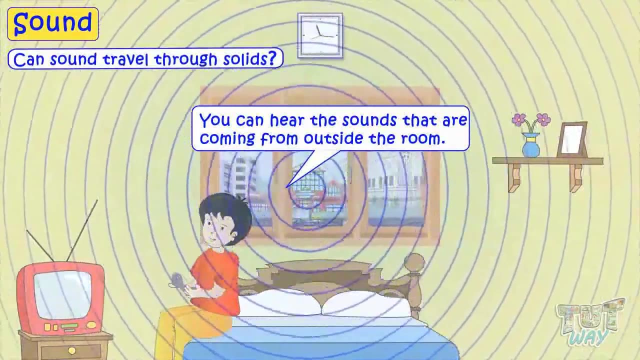 And the ear. So it shows that sound can travel through the solids. If there is any loud noise outside the room, you can hear the sounds that are coming from outside the room. That shows sound can travel through solids. Now let's have a look at a simple activity. 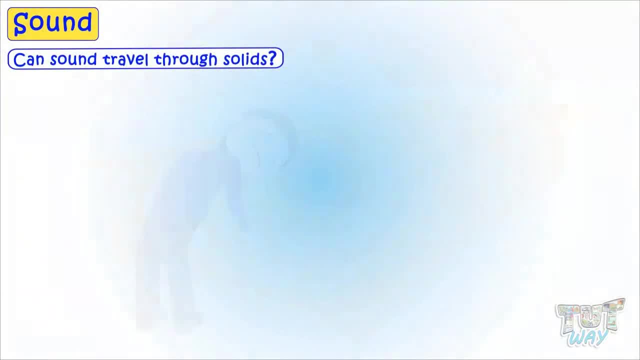 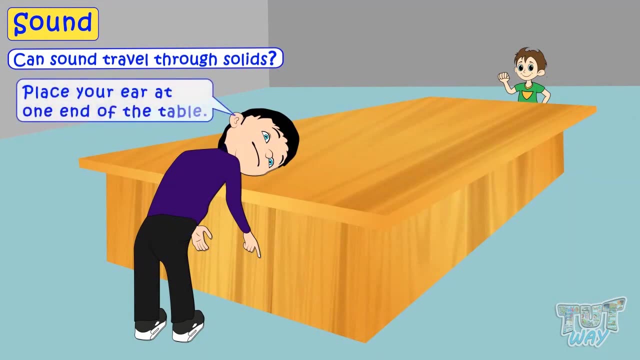 You can also perform the same. You just need a friend of yours for this activity And a table. Place your ears at one end of the table. That can be wooden or metallic. Now ask your friend to tap on the table with his hands on the other side of the table. 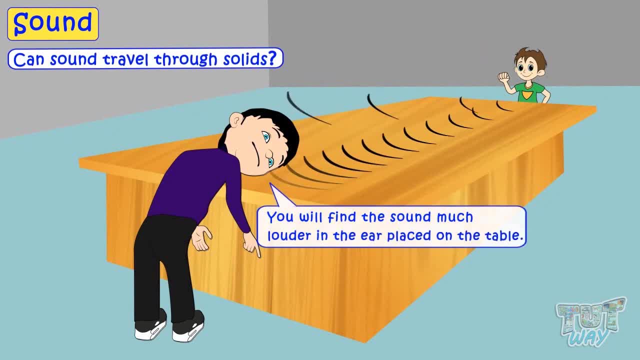 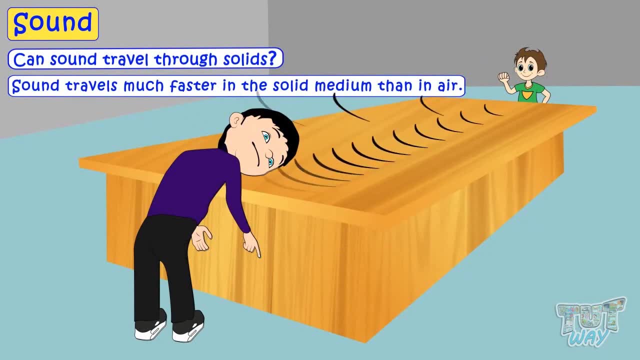 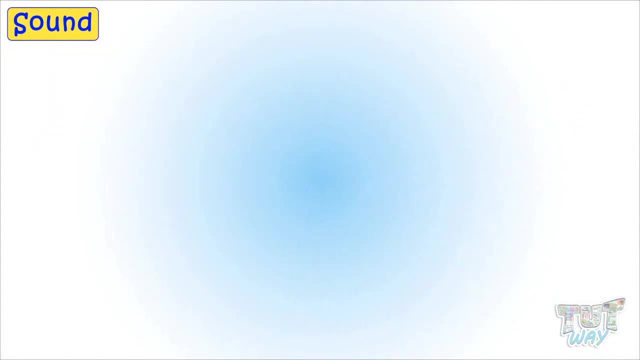 You will find the sound much louder in the ear which is placed on the table. It shows that sound travels much faster in the solid medium than in air. Now let's see if sound can travel through solids Friends, till now we learnt that sound waves originates when something vibrates. 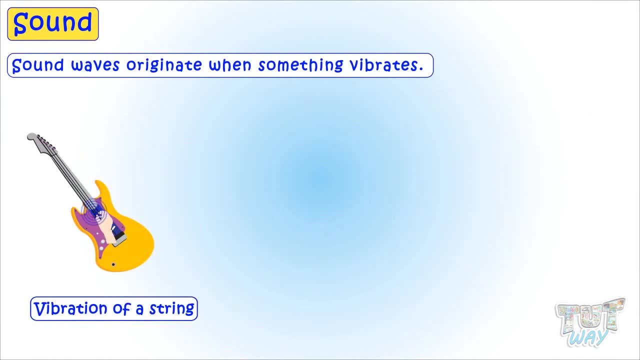 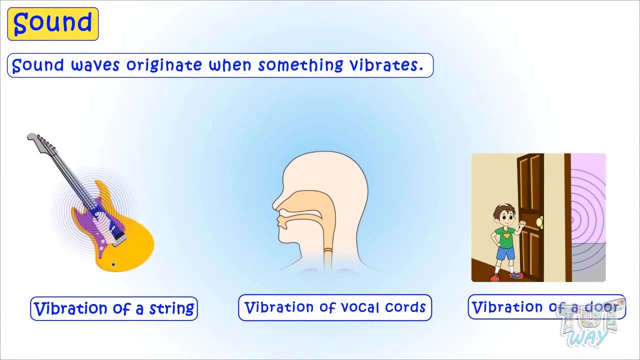 Like vibration of a string of a guitar when it's plucked, Vibration of our vocal cords when we sing or speak, Vibration of door when someone knocks it. Every sound wave originates when something vibrates. Now let's see how this works. 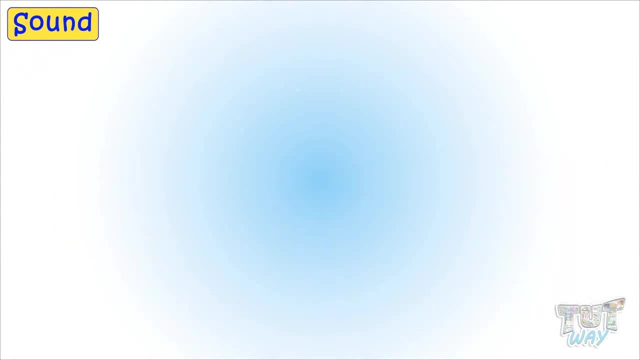 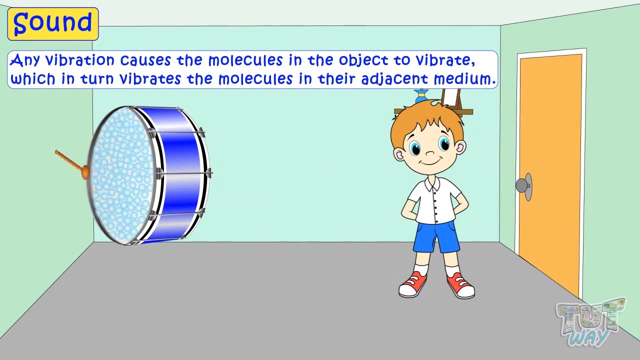 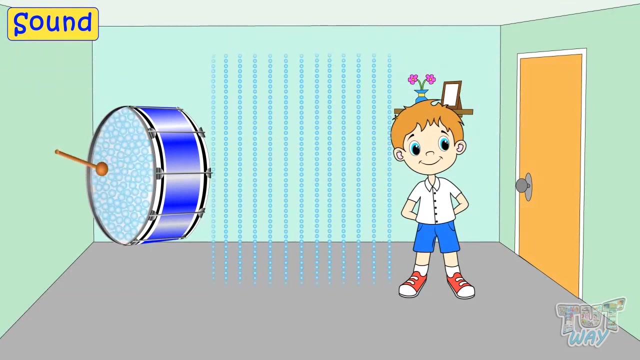 Now let's see how this works. Let's see how this sound wave propagates or moves. Any vibration causes the molecules in the object to vibrate, Which in turn vibrates the molecules in their adjacent medium, Like when a door is knocked. 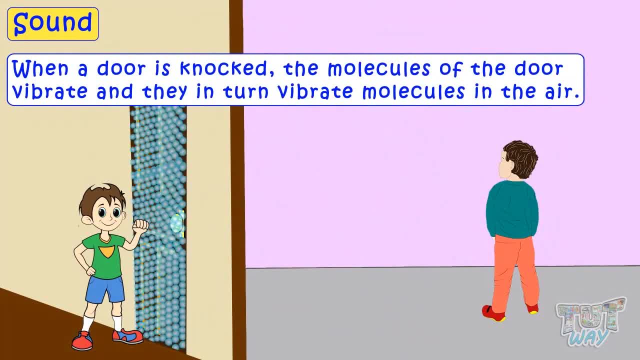 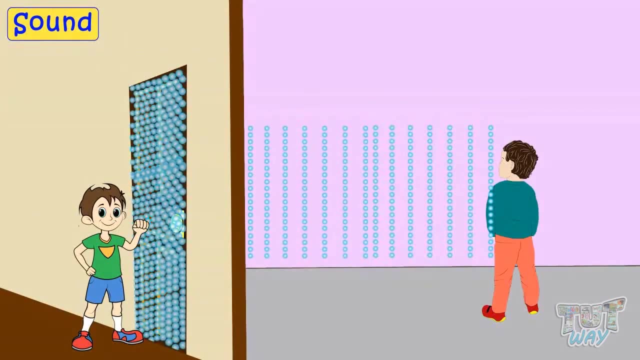 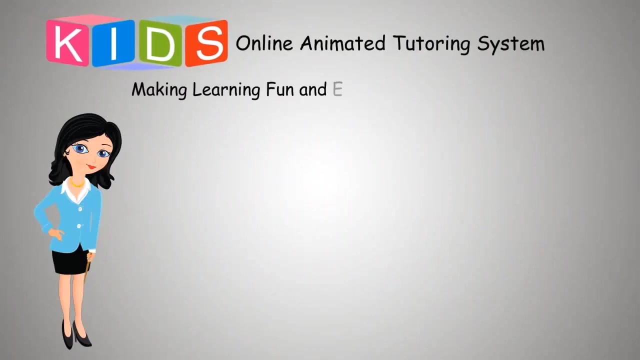 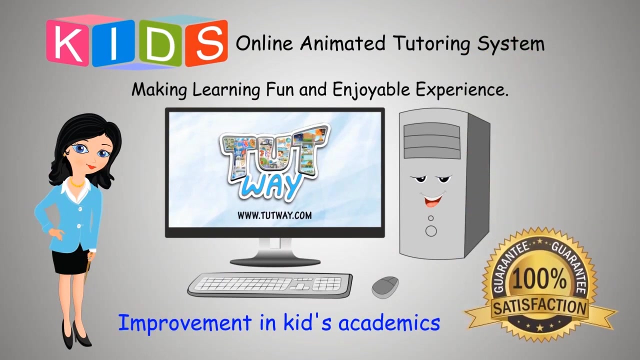 Molecules of the door vibrate And they in turn vibrate molecules in the air And this vibration passes on. This vibration passes on to the next And next molecules And this way, sound travels From the door to the listener. Tootway has thousands of animated videos. 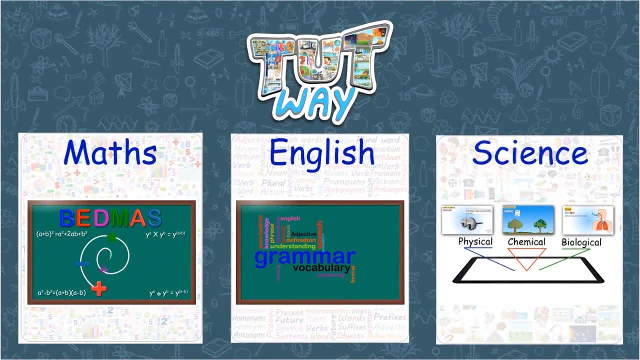 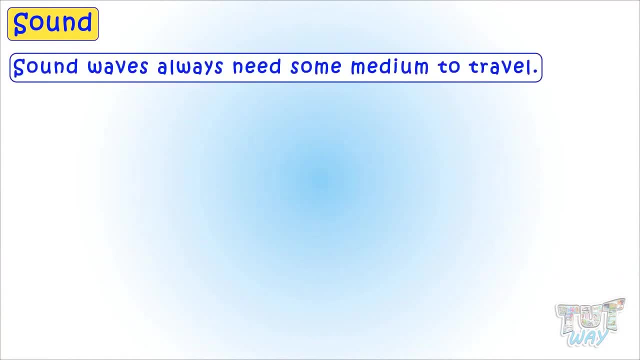 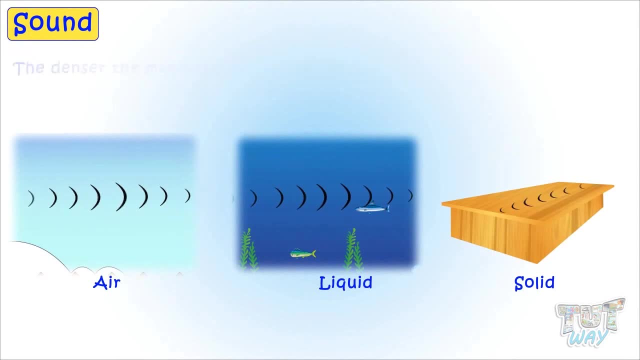 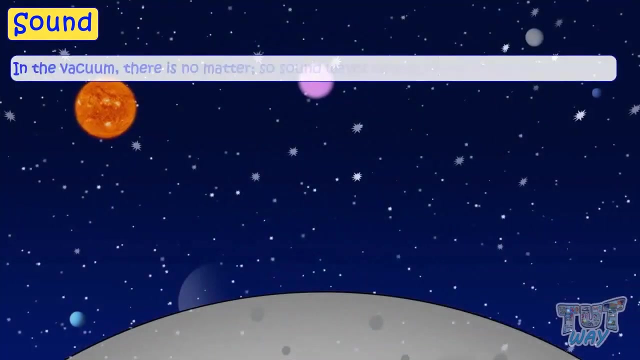 On math, English and science To clear the core basics of these subjects. Sound waves always need some medium to travel. Medium can be air, liquid or solid, And denser the medium, faster the sound waves travel. In the vacuum there is no matter. 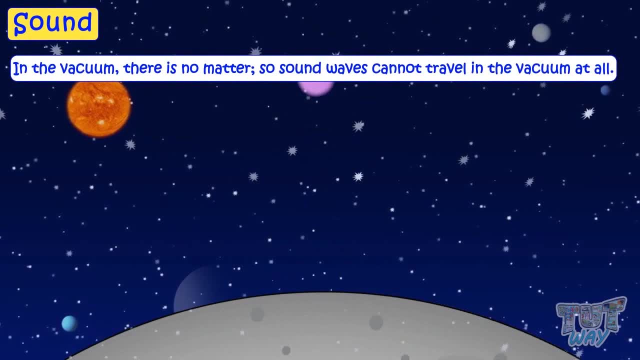 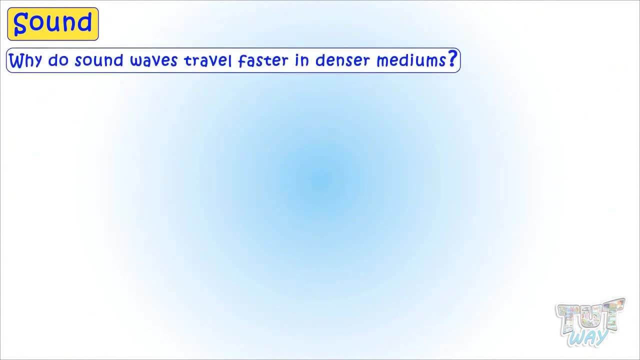 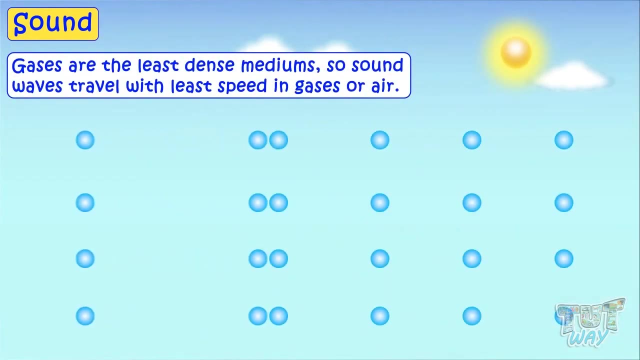 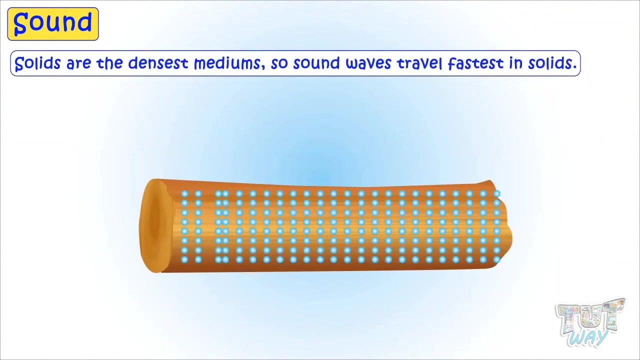 So sound waves cannot travel at all in the vacuum. Now we will see why. do sound waves travel faster in denser mediums? Gases or air is the least dense medium And sound travels with least speed in air. Solids are the densest mediums.